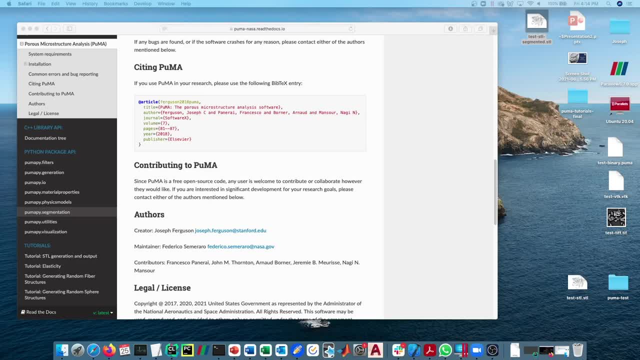 segmentation techniques using things like watershed, machine learning, etc. These may at some point become part of the Puma software, but what I'm presenting right now is just basic threshold based segmentation. So we're going to be using the Puma GUI for this, rather, 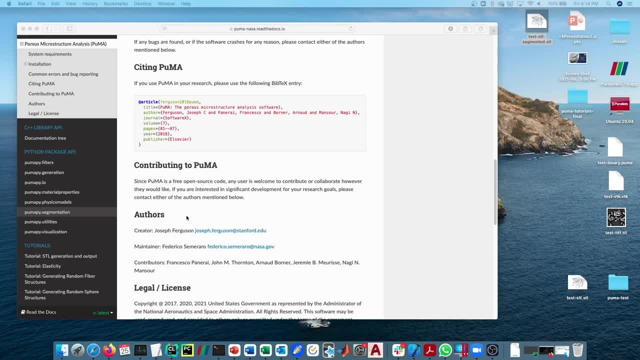 than the Python version. So if you want to use the Python version instead, please refer to the Python tutorials, which are Jupyter Notebook tutorials, and there's a separate video tutorial on how to open and run the Jupyter Notebook tutorials. if you don't know, 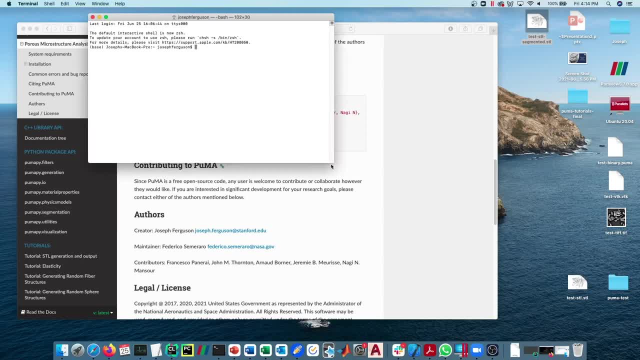 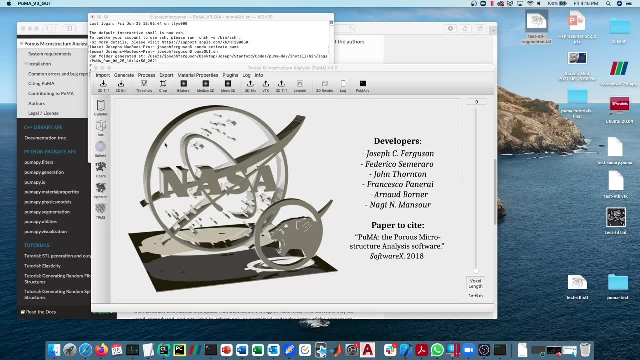 how to do that. So to open the GUI, we're going to open a terminal, type in conda, activate Puma and then type in pumaguish and the Puma GUI should launch. So for this tutorial, we're going to import just a test example of a microtomography. It'll be a small. 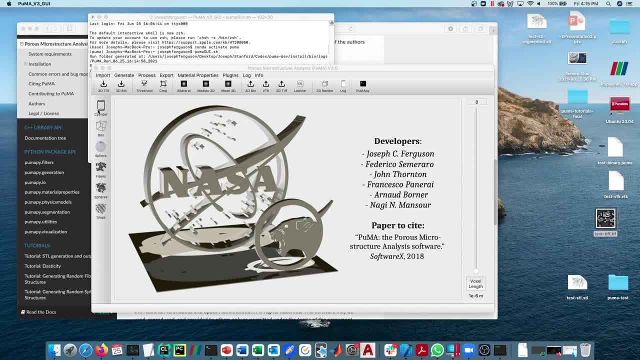 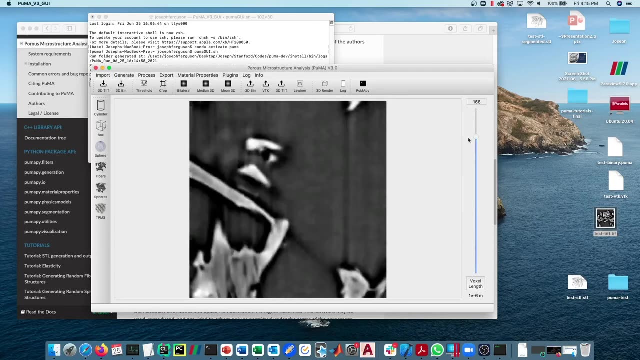 example. So here I'll just drag this in. You can either import tomography using this icon- here You can say import 3D TIFF or 3D binary, or we're just going to drag it right in. So one thing which I've mentioned in other tutorials is that when you import a 3D TIFF, 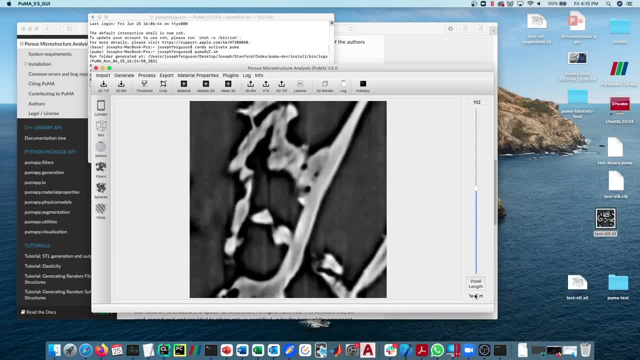 it defaults to a one micrometer voxel length, which, of course, is probably not accurate. So you have to know this value for your specific tomography sample. In this case, the correct value is 1.3e-6.. So we're going to go ahead and update that now. Next, I want to talk. 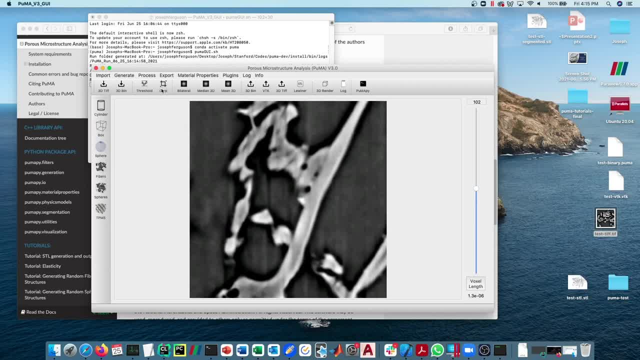 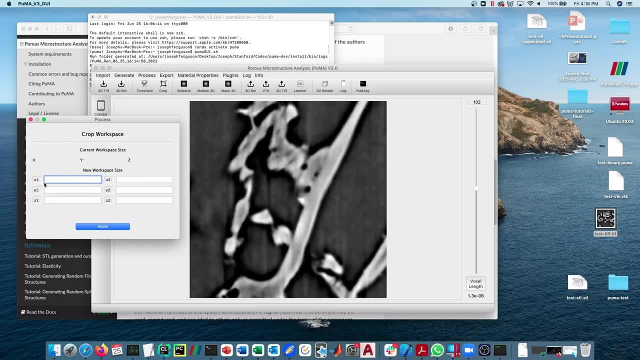 about cropping. Cropping- we use this icon here, or you say process CROP. So, in order to crop the domain, a little window pops up And you're going to specify the new size in terms of minimum and maximum values. Now we are using the C++ indexing and the Python indexing, meaning 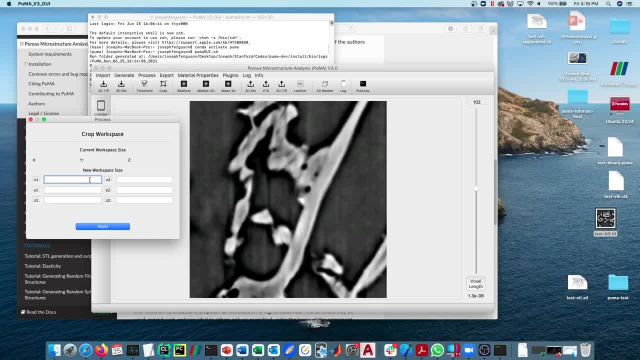 that it starts at zero and it ends at the size minus one. Okay domain here, since this is a 200 cube size would extend from 0 to 199 in each direction and you can see that as we put. the values in this red box will show you. 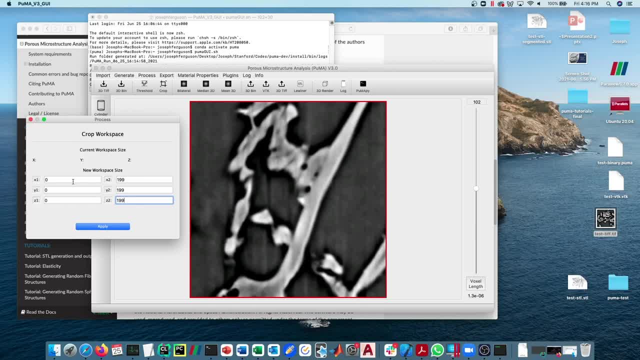 exactly where the new cropped section will be. so if we, for example, wanted to take a section out of the middle, say 50 to 149, then you can see it would select the section in the middle. and if we let's just leave the Z direction as 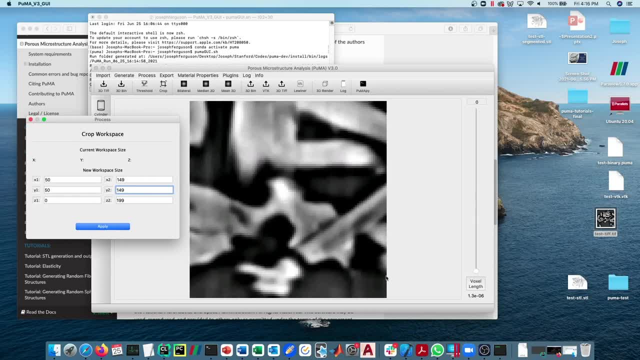 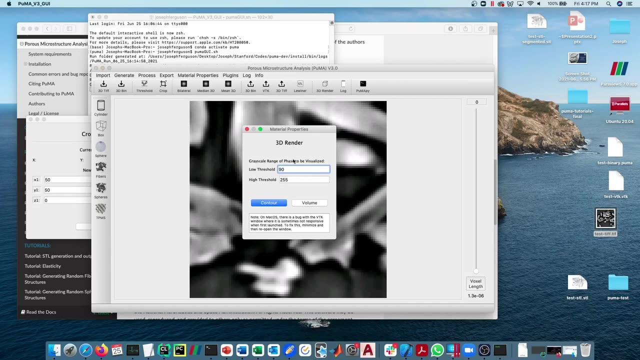 full 200. so now if we say apply, then it will have cropped the domain to be now 100 by 100 by still 200 in the Z direction and if we visualize that so 3d render select our cutoff range, which we'll all talk about this in the 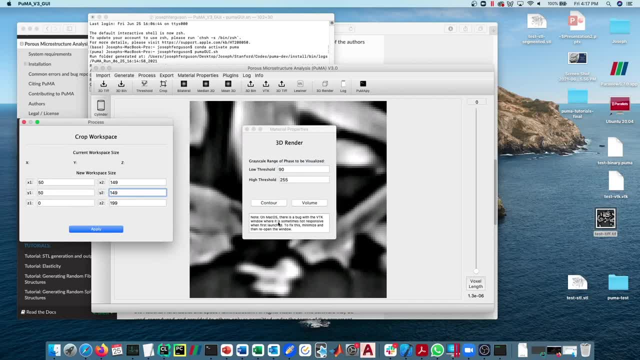 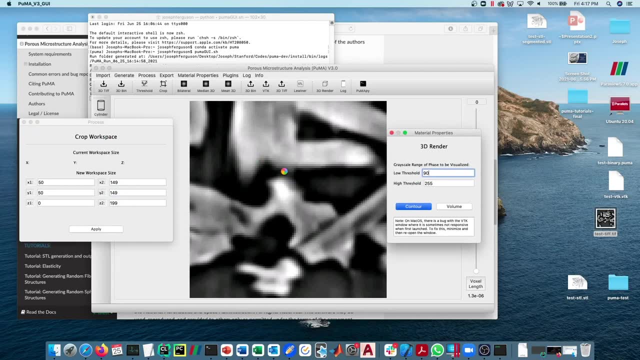 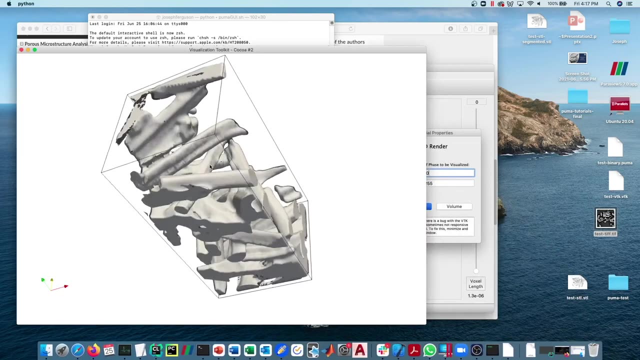 segmentation section. but for this tomography 90 to 255 is a good cutoff for the material. generate a contour and you can see the domain is is: uh, the domain is rectangular now, so it's been cropped in the X and Y direction, but left alone in. 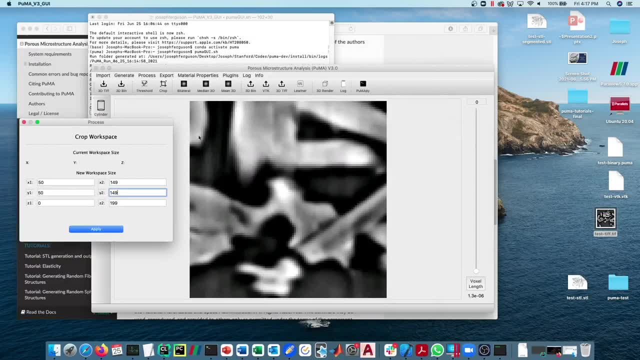 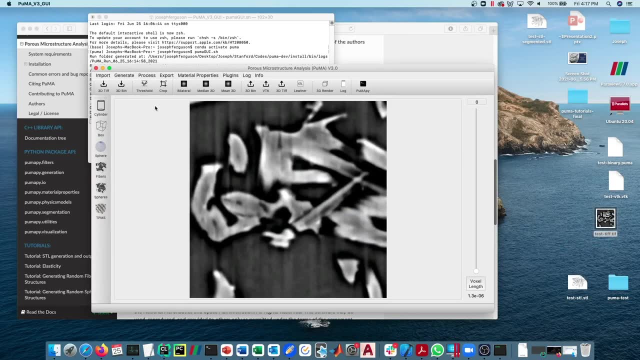 the Z direction. okay, so let's go back to the original TIFF. I'm just going to drag it back in there. and now we're back to the 200 cubed example. and now we're going to talk about thresholding. so we're going to talk about thresholding. so 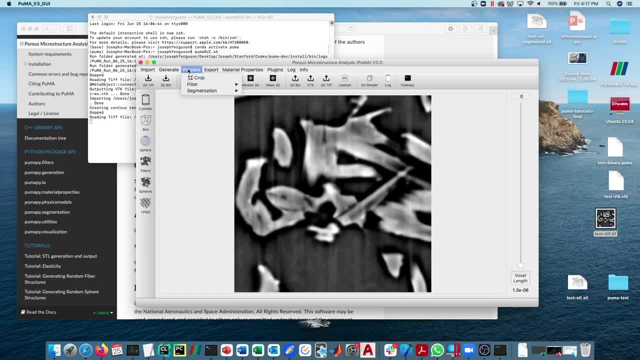 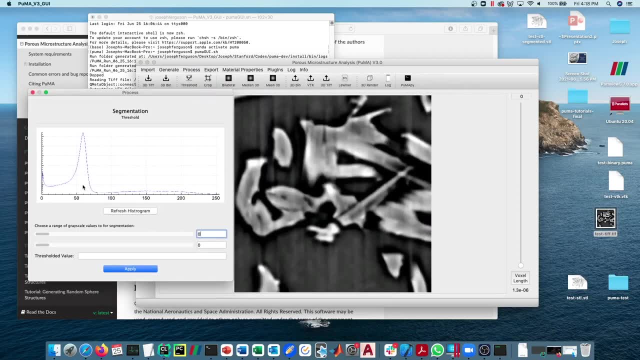 if you click on this threshold button here or you go to process segmentation threshold, what will pop up is a histogram of the grayscale values. so typically, if your material is two phase, then you're gonna have two peaks, and it's worth mentioning that this peak here at 0 is usually just a. 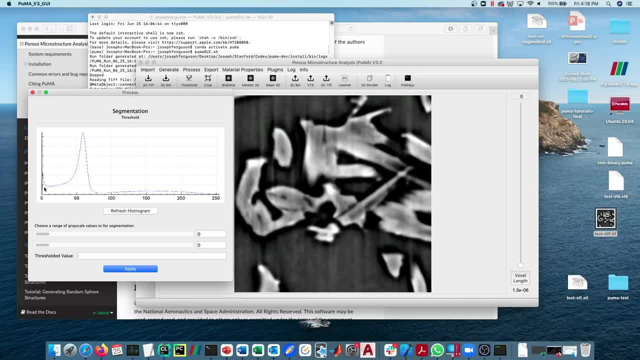 visualization artifact. artifact and is not actually represent its own distinct material phase. but this peak here is the height of the text, faster than our model wanted to be stable and so around 60 is kind of the most probable value of the void phase here. and then you can see this second peak which is quite elongated here is kind of here in: 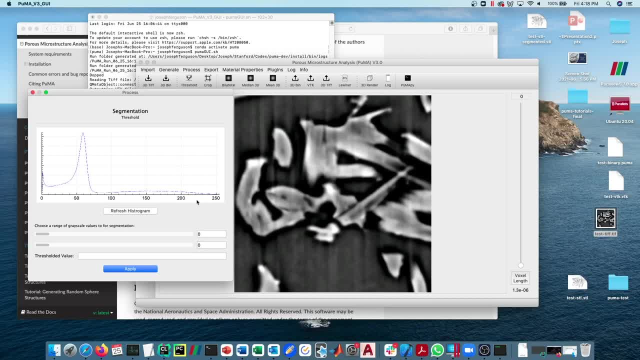 the middle. maybe around 170 is the most probable grayscale value for a solid carbon in this case, since this is a carbon fiber material. so choosing the appropriate threshold value is usually a bit more of an art than a science. it can be tricky depending on the material. sometimes simple thresholding does not. 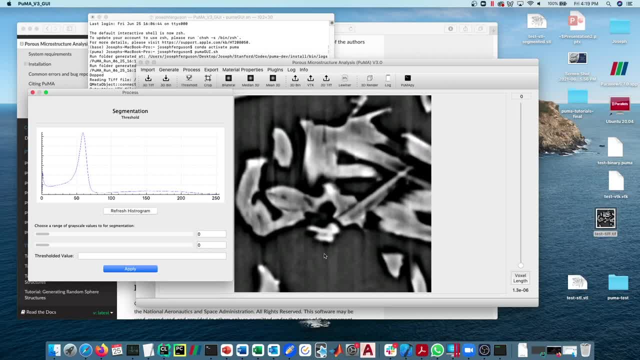 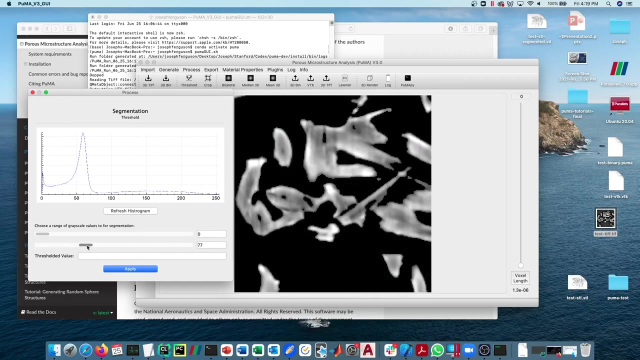 do a very good job. filtering can help, but often more advanced segmentation techniques are needed. so if segmentation, threshold based segmentation- is not working for you, it may just mean that you need to apply more advanced segmentation techniques to this. so the way in puma that you can look at just simple thresholding, you can move. 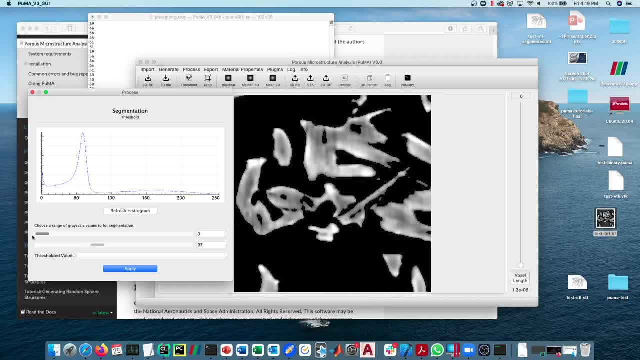 these scroll bars to select maximum and minimum values for a, for a given section, and then that new section is going to be applied here in this visualization, a new value which defaults to zero, but you could, for example, if you wanted to visualize the solid phase, put that to. 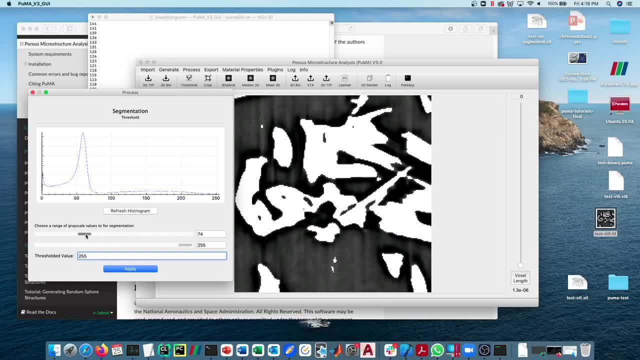 55, for example, and then you can move these sliders around in order to see how well, how well this range is doing to capture the material. now, in this case, this material segments very well at a grayscale value of 90. so if we were to want to segment this, anything between 0 and 89 is void. anything between 90 and 255 is solid. anything between 90 and 255 is solid. anything between 90 and 255 is solid. 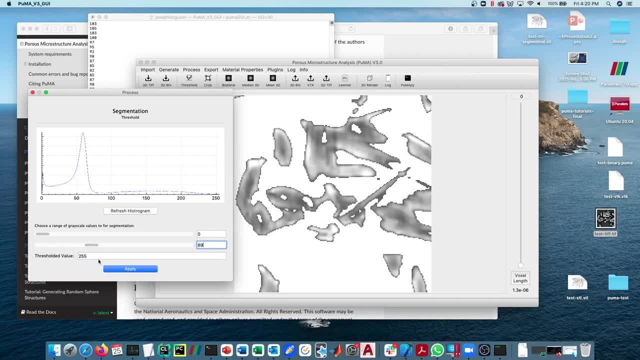 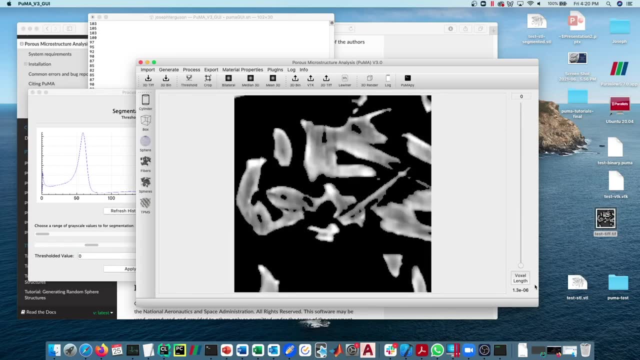 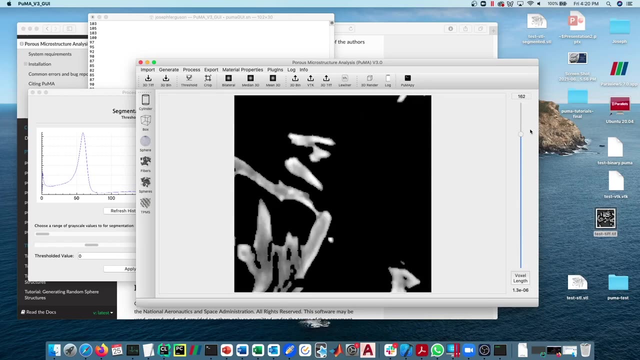 we can go from 0 to 89 and set that to have a grayscale value of 0, and if we click apply, then now, as we scroll through, we can see that that's been applied. so now our solid material actually still has the grayscale range in it from 90 to 255, but the void phase has been zeroed out here. so typically 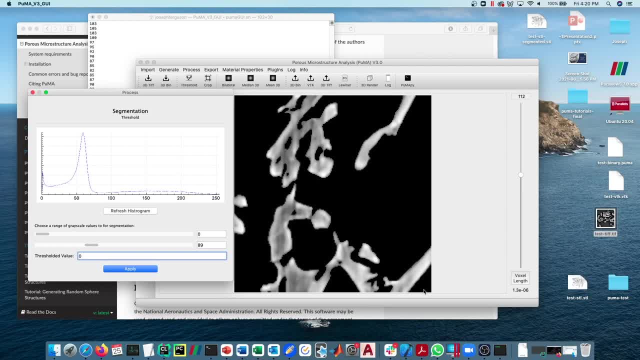 speaking, when you binarize an image you're going to want to have, you know, 0b void, maybe 1b your solid, and if you have multi, multiple, different phases, you can have it be 0, 1, 2, 3, etc. so let's go ahead and do that. we can say: 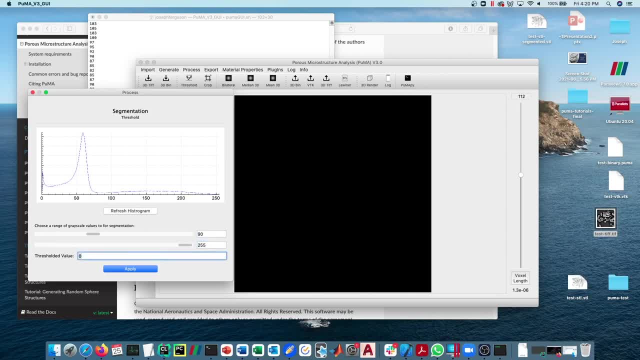 anything between 90 and 255. we're gonna assign a threshold value of 1. now, with our current visualization here, we kind of have it hard-coded to an 8-bit scale. in future updates we're going to change that so that the so that the